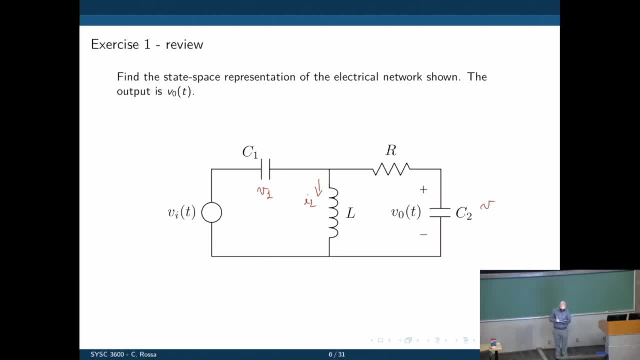 as another state variable And we can define the current, the voltage across the other capacitor as the third state variable. So we can define our vector of the state variables X as X1, X2,, X3, and this is going to be V1, IL, V2.. 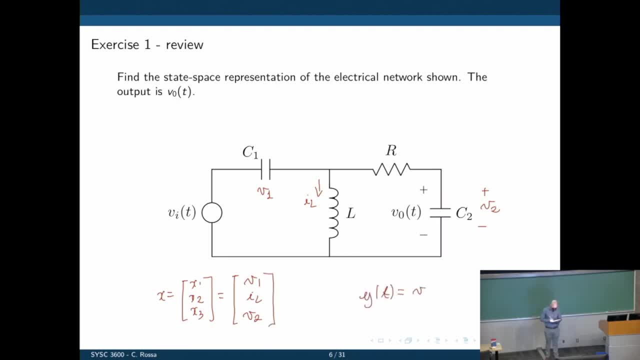 The output of our system is V0,, which turns out to be V2,, which shows that to be V2.. Let me just check here with my notation So I follow the same. Don't make a mess, Yeah, Okay, So let me copy here the variables we defined here. 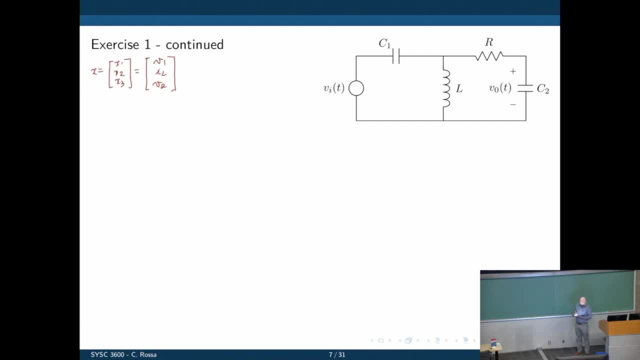 And we have V1, IL and V2.. Okay, Now that we have the state variables, we can start to write these equations of this system. But before we jump in to write these equations, let's think about what kind of equations we need. 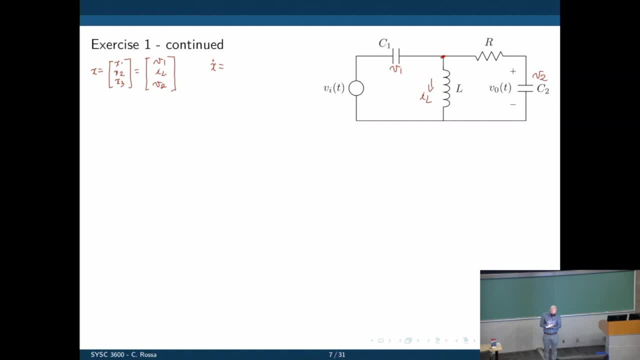 Remember that for the state space representation we need: X equals to AX plus B, B. that's supposed to be a B B times U. Now look at this equation. here We have the derivative of each state as a function of other states. 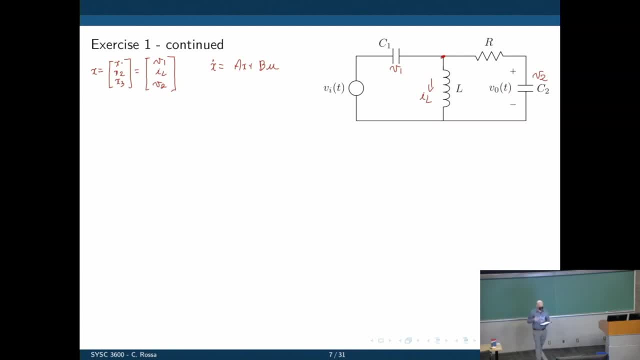 not their derivative as a function of other states. So we need equations That have in them the derivative of one state, the derivative of each state. one equation for each state. Let's look for these equations that way, rather than going ahead and writing all the equations. 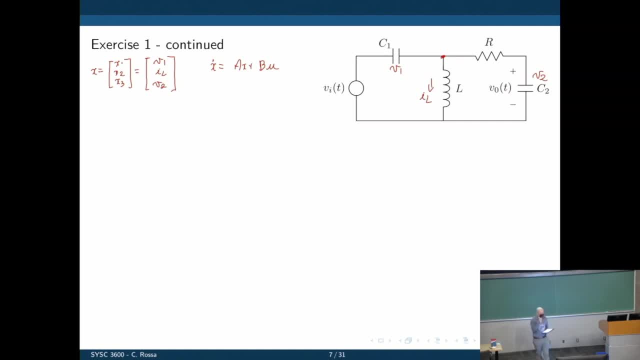 and then figuring out what to do with them. We know that we want the equation to be in this format, So let's look for derivative of states in our equations. Let's start with perhaps that point over here, This node A. We know that the current going into node A, 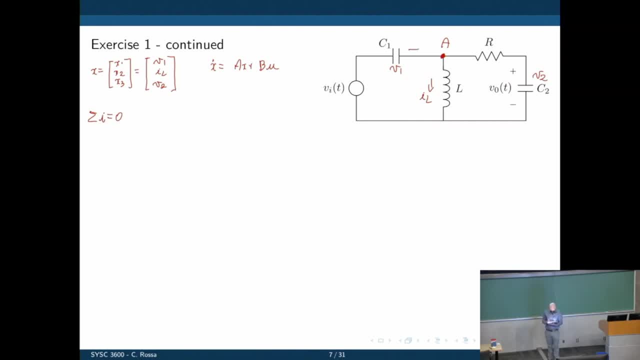 is sums up to zero, And the current going in node A is the current IC plus current IL plus current I2.. Right, all currents going in equals the sum of currents going out. Now, why did I pick point A? Well, because if you want to express 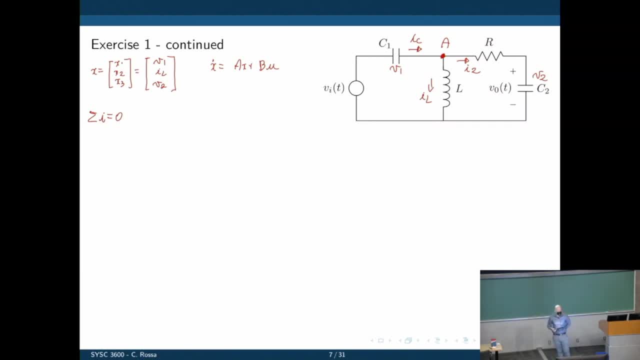 the current through the capacitor. what is it? Is this? it's C times DV1 DT, isn't it? The current through the capacitor is C times DV1 DT, And that's already the derivative of one state. All right, so we are on track here. 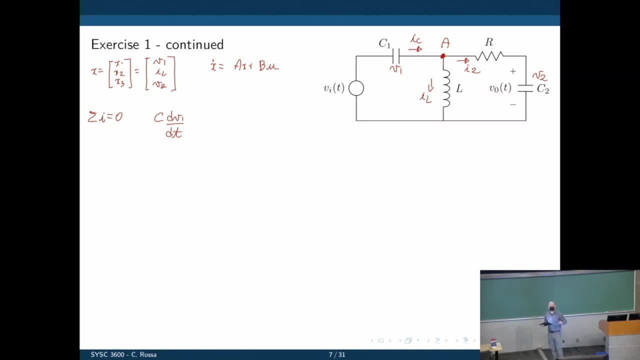 to find the first equation we need, because it already includes the derivative of one of our states. And what is this equal to? DV1 DT, which is the current IC. What is this equal to? What is IC equal to in terms of current? 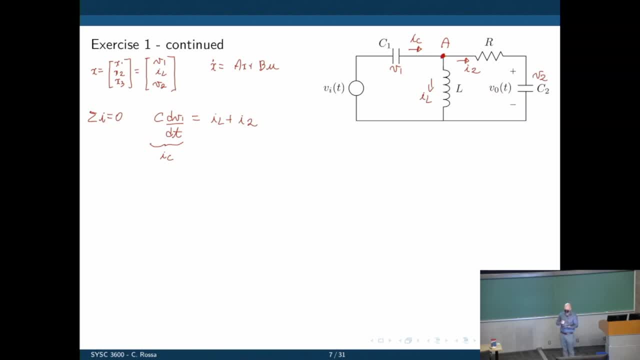 Plus I2.. Yeah, plus all currents coming out. So that's right, which is also good, because here we have already another state variable, IL, But I2 is not a state variable. I2 is just an internal variable. We have to get rid of it, because- look at our equation here. 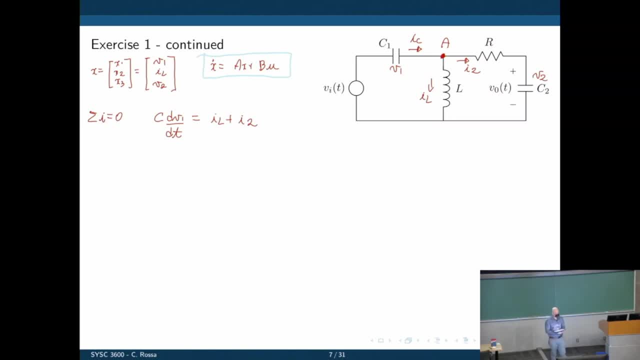 Our equation only takes state variables in them. I2 is not one of our state variables, So we need to replace it. How we're going to find a equation to replace I2? That's only a function of state variables. We have basically three options to find equations here. 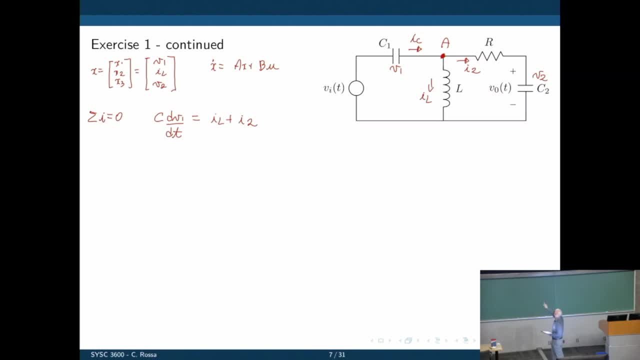 We can do each loop, the first loop, the second loop, or we can do the outer loop. Which one would give us the result we want? Let's think about it. If you do the first loop, that doesn't help, because I2 is not even there. 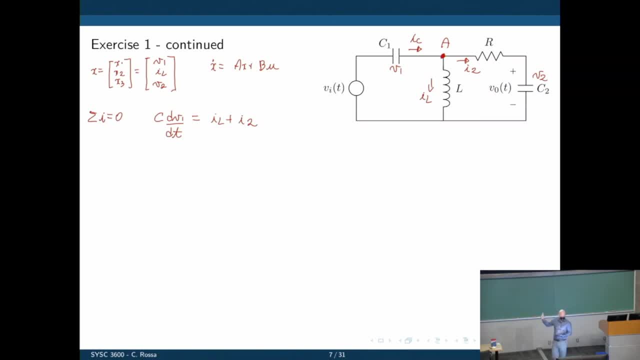 If you do the second loop, what happens? We have the voltage across the capacitor plus which one I2.. Which is a state variable. We have the current through the inductor, We have the voltage through the inductor and we have the voltage across the resistor. 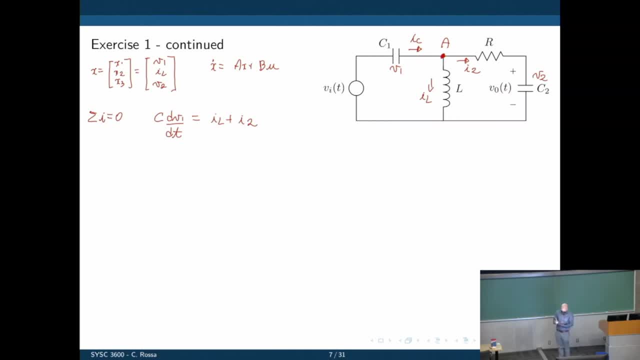 If you do this loop here we have V2 plus I2 times R plus LDIL DT Plus DIL DT, and that's the problem, because you're now introducing the derivative of another state And you cannot have that in our equation. We want something that is only function of state. 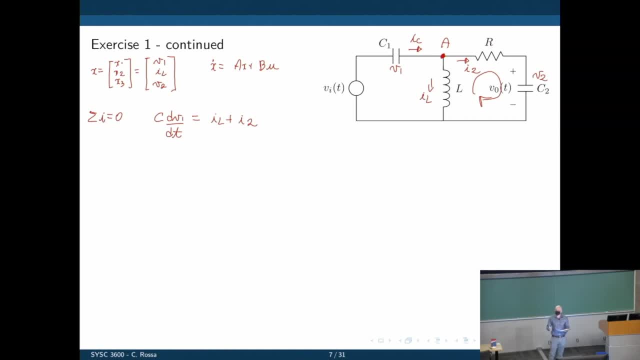 not their derivative. So you see why that function doesn't help us at all And because if you do that loop, we are introducing another derivative in the equation for I2, and that is not going to help with solving the problem. But let's look at the outer loop. 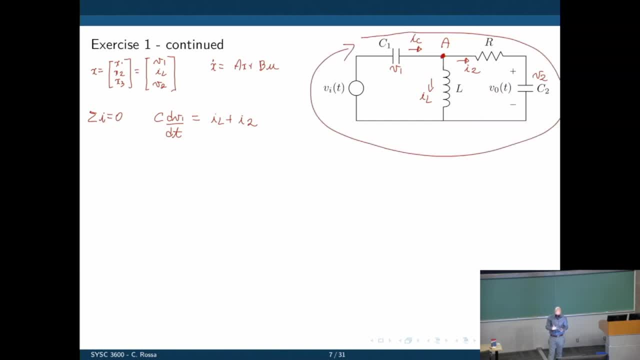 If you do the outer loop here, what do we get? We get this, We get: the VI is equal to V1 plus I2R plus V2.. You see, this equation is a lot nicer because it only depends on the states and only depends on the inputs. 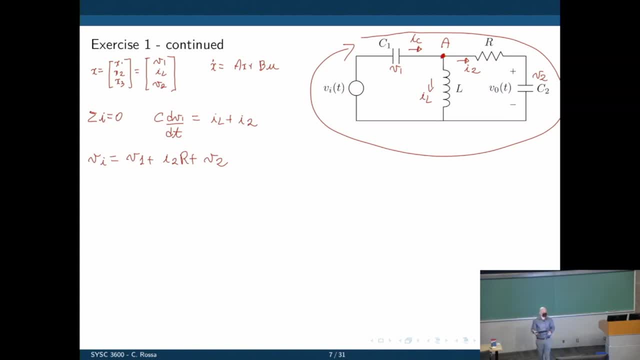 And you can now solve for I2 and then replace that in the previous equation. And you wouldn't be able to accomplish that with the inner loop equation because that has a derivative of a state in it. So this isV2 over I2.. 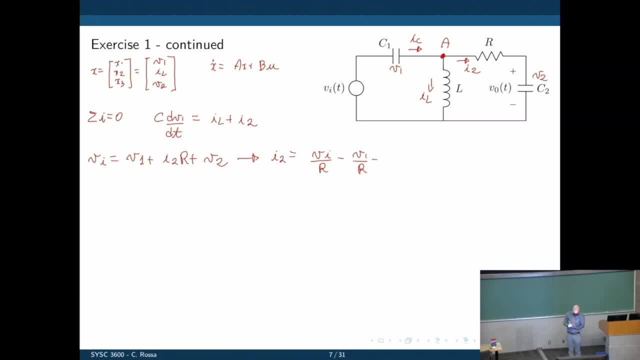 Are you okay? up to here? Yeah, gonna replace So for I2 and I2 is VI over R, minus V1 over R, minus V2 over R. And now this replaces I2 over here. So this is the V over R, So this is the V over I2 again. So this is one of the spin points. 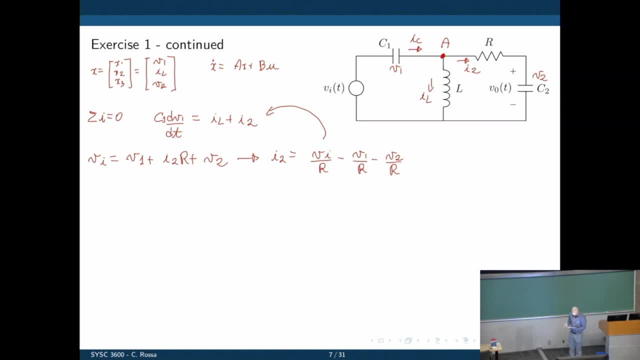 T one right. So we have now. now let's write that equation C one and D V one over D T equals to IL plus V. one V R times PI times R minus V. one times R minus V. two times R. Good, so we have now the derivative of one state. 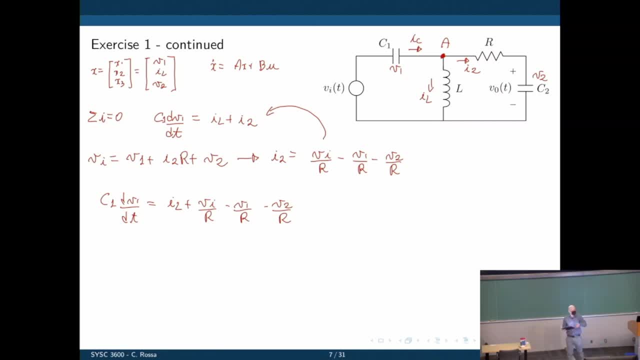 as a function of all other states, Of other states and the input. Now we can write our equation as a function of the state variables. What is D, V, I, D, T as a function of our state variable? D V one, D, T as a function of the state variable? 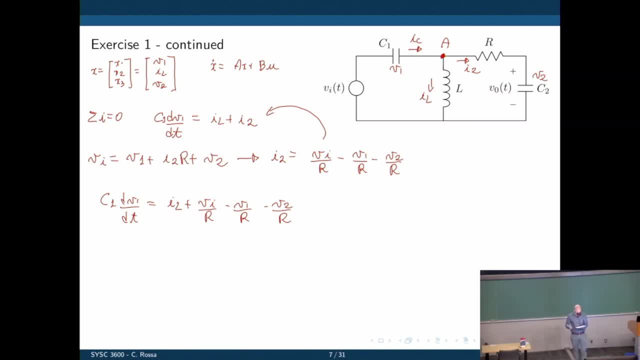 V one is X one, So D V one, D T, that's X one. dot. That is equal to IL. IL is X two. VI is the input that doesn't change. V one is X one and V two is X three. 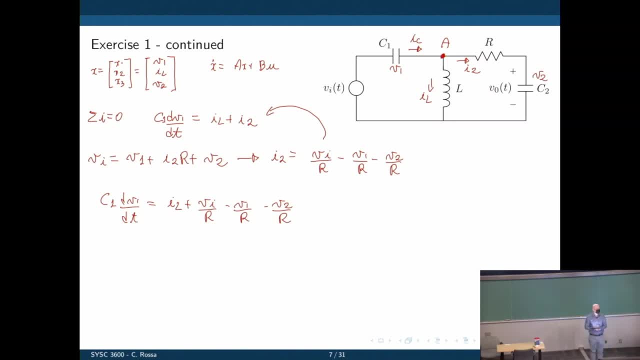 Does that make sense? So sorry, I can't hear you. Oh yeah, Sorry, I accidentally pause it. Does that make sense? Yeah, Okay. So here we have the first equation for our state-space representation. So I'm going to move this to the side here. 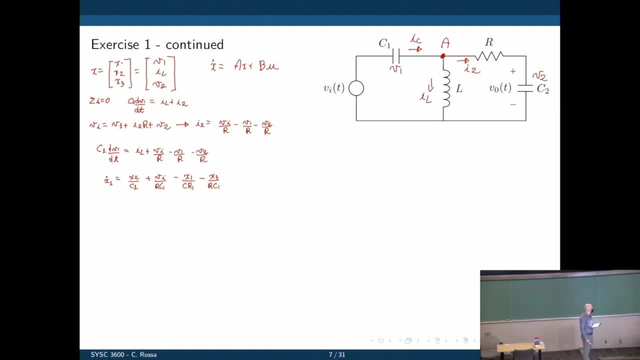 Can you guys still read it? Yeah, And now let's look for another one. And what can we do for the other one We can look at? let me see What did I do here. Okay, Now notice how we got here the derivative of V1,. 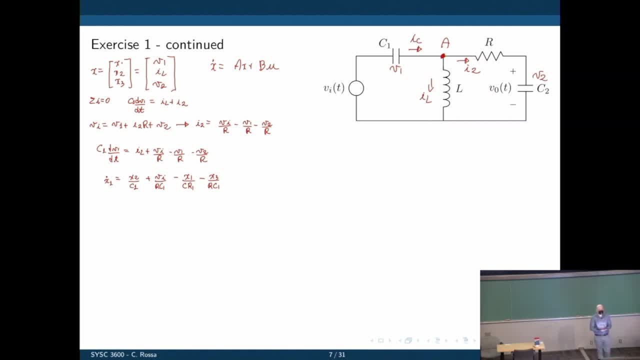 the derivative of X1, was to look for the current across the capacitor C1. So we can do the same for capacitor C2.. And you can write for capacitor C2 that I2, equals to C2, dV2, dt. 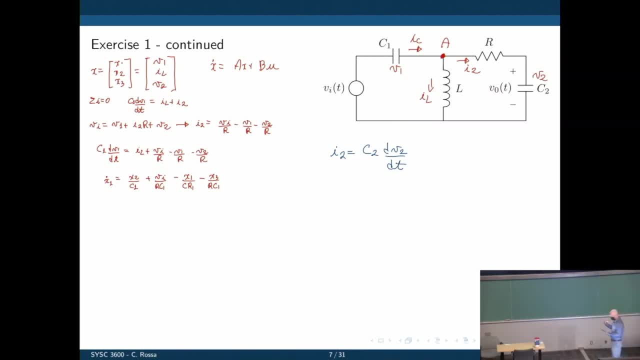 And that's how we got the derivative of state X3.. Now what is I2?? I2 is not a state variable, So we need to replace that with a function of state variables. And here is the equation we just derived for I2.. 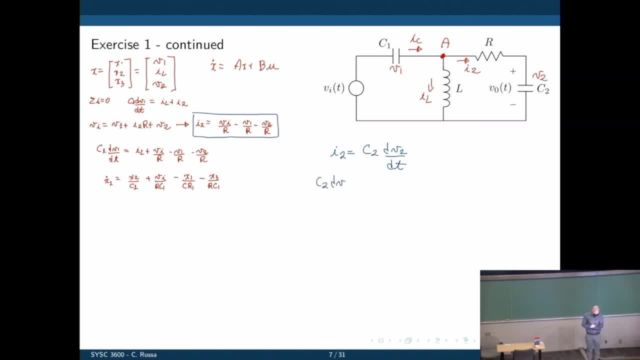 We can use that then. So C2, dV2, dt is simply VIR, VIR minus V1 over R, minus V2 over R, By simply using the equation for I2.. And now we can rewrite this equation as a function of our state. 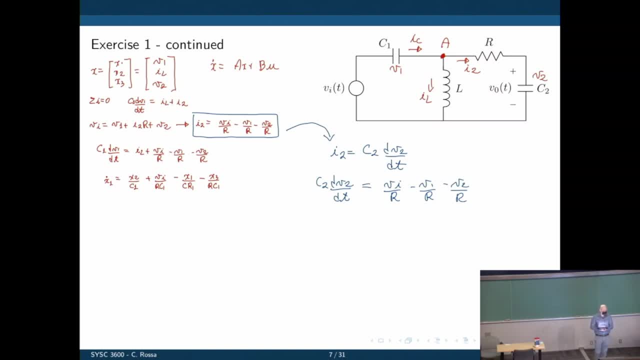 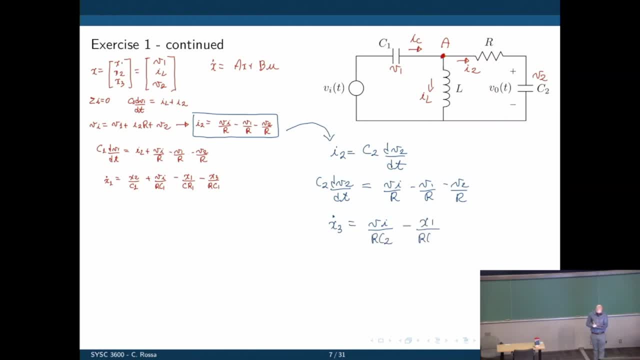 That's V2.. That's V2.. That's the input. V1 is X1.. And V2 is X3.. And here we have now the second equation. Here is the first. That's the second equation for X3. now, 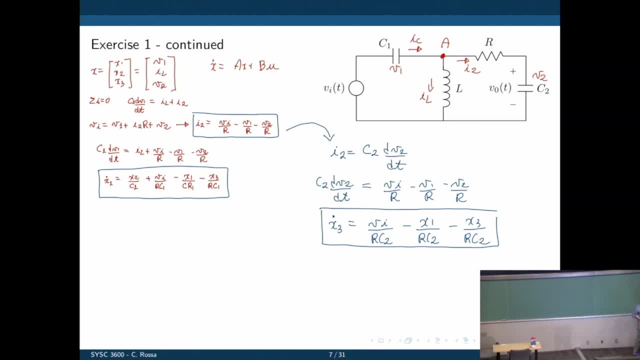 We are missing one equation. We are missing the equation for X2 dot And the equation for X2 dot. Now we need to find an equation that gives us the derivative of the current in the inductor. We are looking for the derivative of X2.. 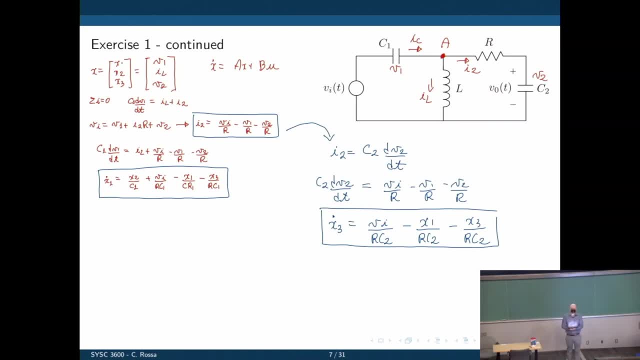 X2 is IL. So we need a equation. So we need a equation that explicitly has in it the derivative of IL. Where do we find that equation? Where do we find that equation, The equation that gives us the derivative of IL in it? 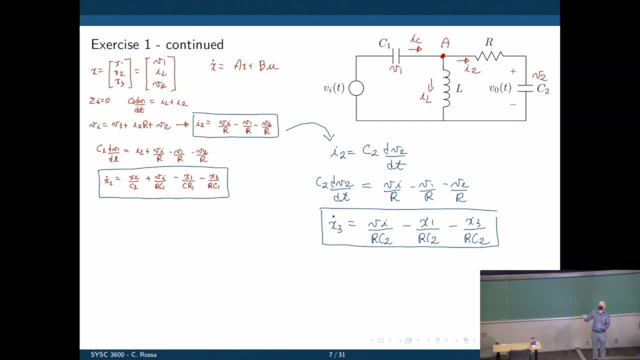 I'm insisting on this because typically students just go ahead and write all the equations they want And then they get stuck. So before we jump and write all the equations, think about it. Which equations equation do I need? In this particular case, we're looking for the derivative of IL. 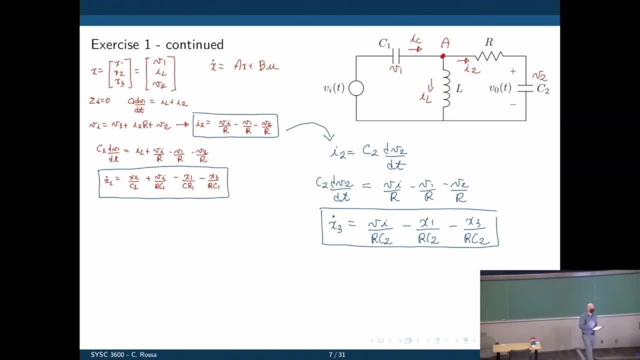 We need an equation that it gives us in the equation the derivative of IL. Where can we find that equation? IC minus I2.. Yeah, we already use that equation to some extent, So we would be kind of repeating it, Right? And if you do, IC minus I2.. 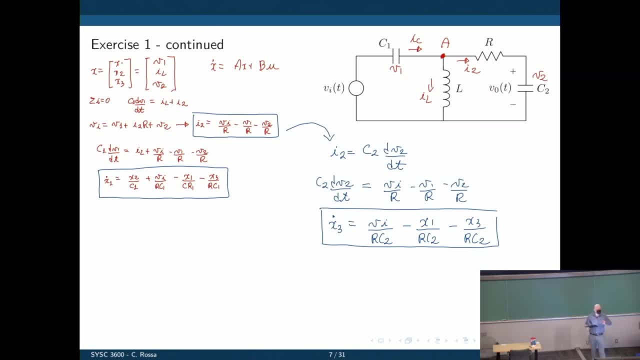 Right, That is IL. It's not the derivative of IL. So that doesn't work. Right, That doesn't work. Yeah, Aha, Right, Very good. So we do this loop Basically. Right, We do this inner loop. 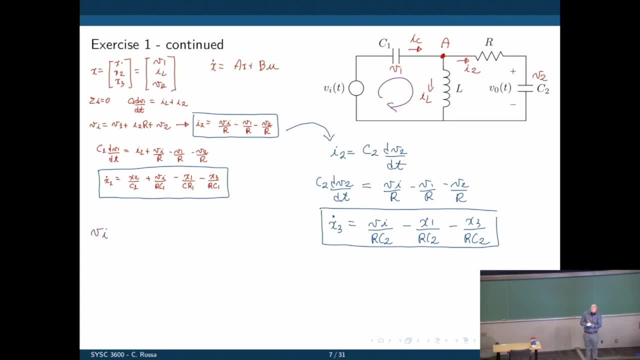 And in this inner loop we have VI equals to V1, plus Plus L- DILDT. Perfect, Look at this. We have a input and we have a state variable and everything else. And then the other term is IL that we were looking for. 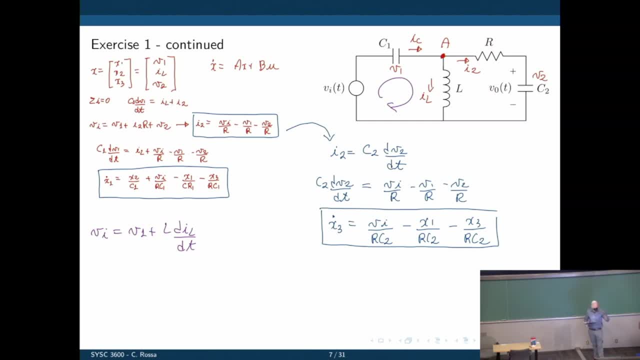 Right. So the equation doesn't even need any manipulation. It's ready in the format we want, And now we can write this as a function of the states. X2 dot, which is DILDT, is equal to VI over L minus X1 over L. 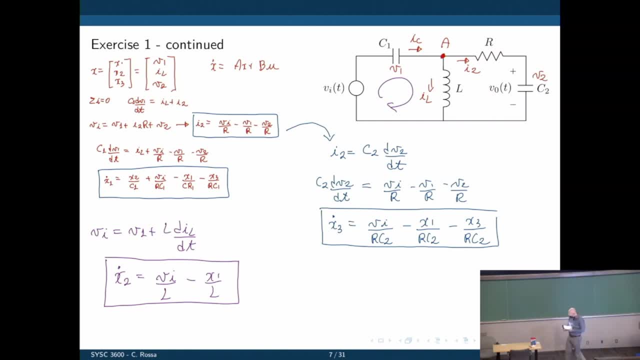 Okay Now. so when you have to solve this problem, think about the equations we saw in the beginning there. Where will I find the derivative of these states? It starts there if we're writing the equation that explicitly showed the derivative of a state. 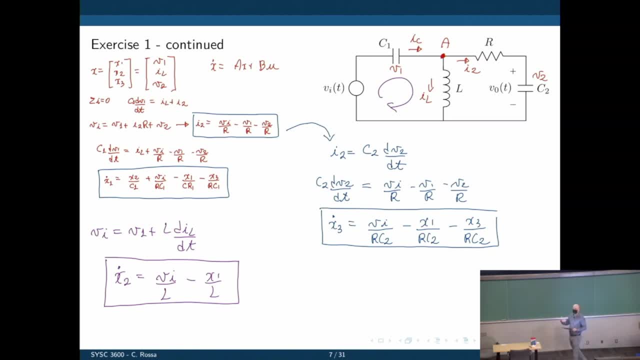 And then, if you end up with variables that are not state variables, replace them with other functions that are state variables by finding an alternative equation. Are there any questions? so far, No, Okay. so this is really the problem. now is solved. Now we found the equations. 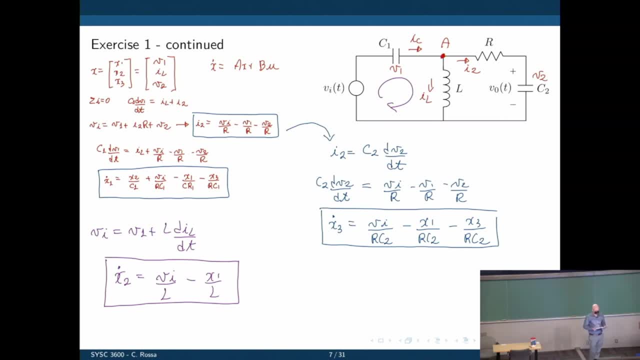 now need to rewrite them as a matrix. I'll give you some time to take notes and then we'll move on. All right, So now we're going to solve the problem that we saw in the beginning there, And then we'll move on to the next problem. 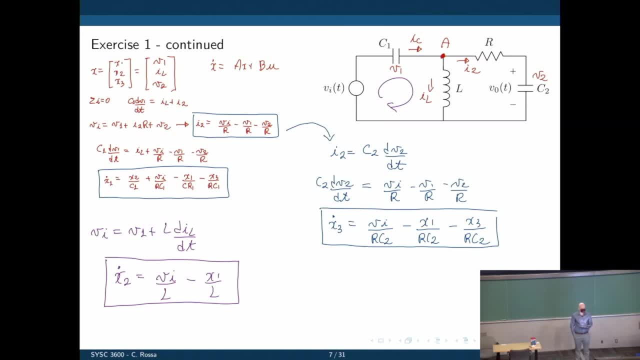 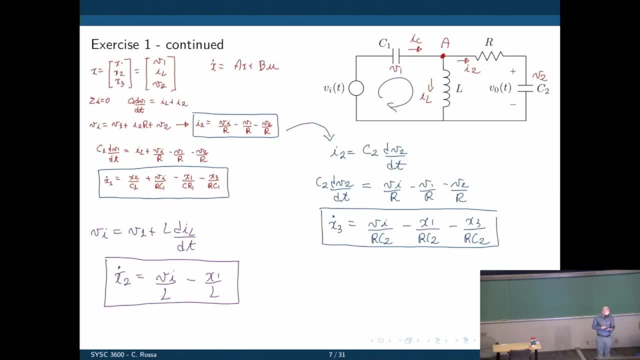 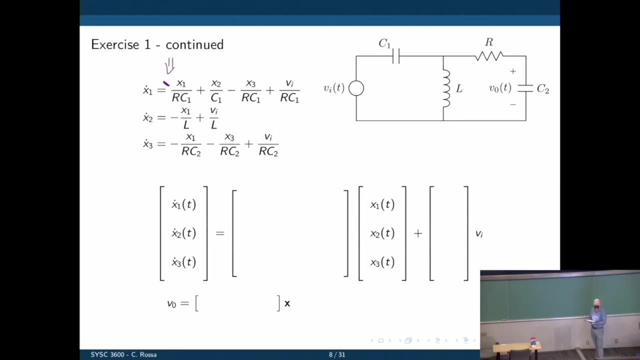 Is X one. there's a negative sign missing there for X one dot minus. yep, X one dot has a negative sign here. Yes, yeah, there's a negative sign missing. Please add it there. Okay, so we want the equations now to be written. 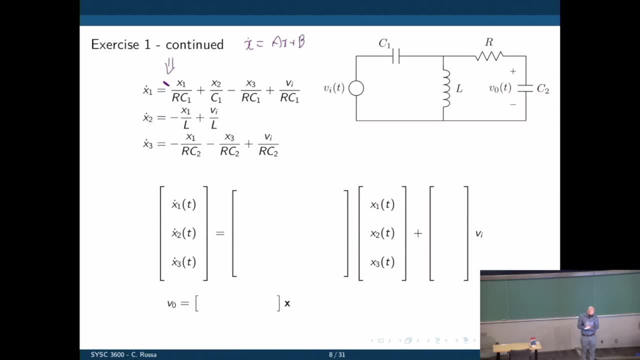 in the form of X dot equals to AX plus BU. U is the input. Here's the format: X, one dot, X, two dot. X three dot equals to A, is the big matrix, X, B and the U is simply VI, the input. So what goes in the first row of A? 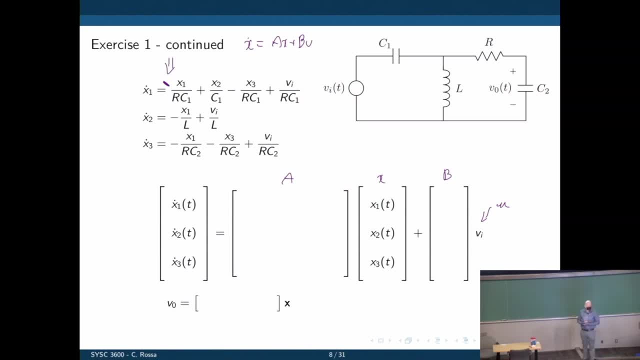 While we are dealing the first row of A, you are dealing with X one dot. So you're going to put there all coefficients of the state variables X one, X two and X three. So the coefficient for X one is negative. 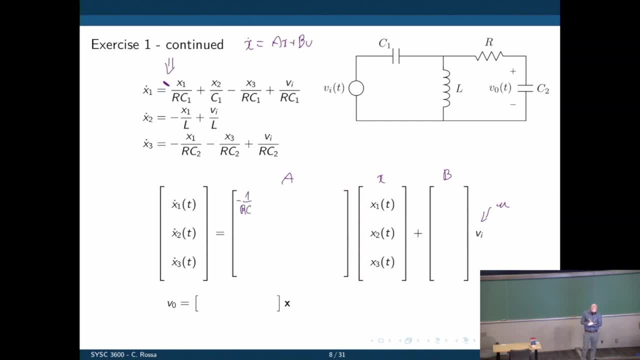 So the coefficient for X one is negative One over our C one. the coefficient of X two is one over C one. The coefficient for X three is minus one over our C one, And the input here shows up in the equation for X one. 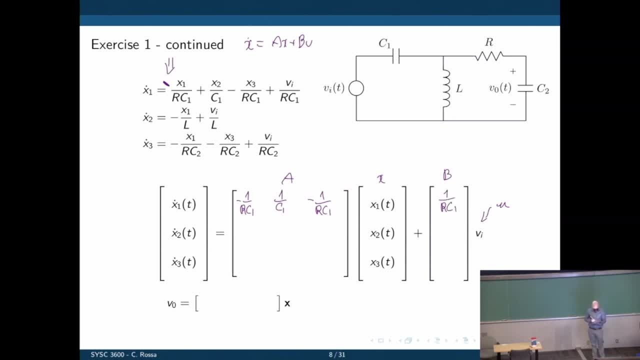 and is multiplied by one over our C one. Now, looking at an X two dot: X two dot has X one in it. The coefficient is minus one over L, Doesn't have X two, doesn't have X three And VI is there in. the coefficient for VI is one over L. 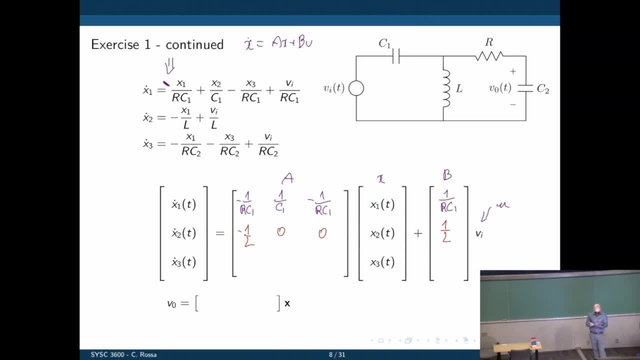 And finally, we have X three. What are the coefficients for X three dots? Excuse me, X three dots? We have negative one over RC two for X one, zero for X two and the same negative one over RC two for X three. 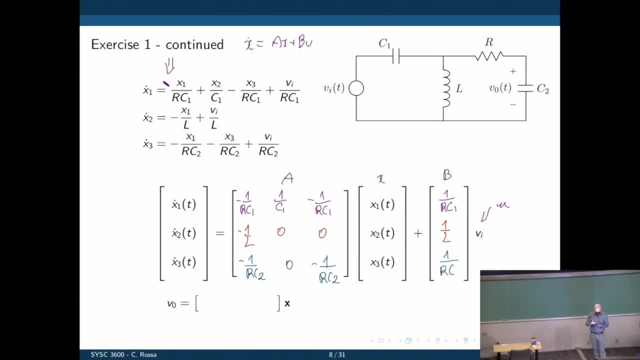 And the coefficient of VI in. there is one over R times C two. Now notice that if you multiply this out we go back to the three equations we started from. I use a simple linear algebra here, just multiplication of matrices. But that's half of our job. 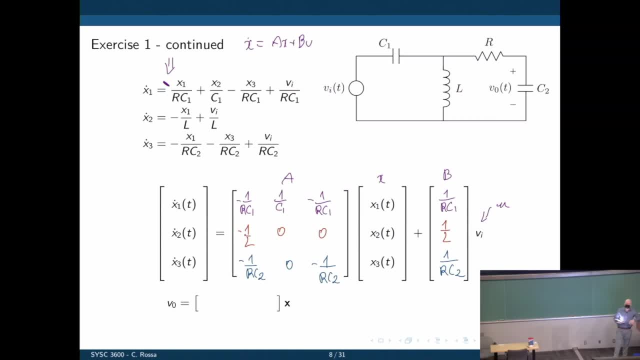 That's one of the equations. We still need another equation. That other equation is the equation for the output, And we define the output to be V zero. We chose it to be the voltage across the capacitor. All right, it turns out to be V zero. 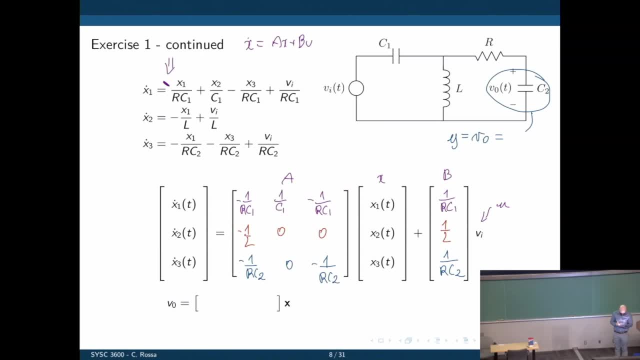 So Y equals to V zero, which is the same as V two, which is X three. The voltage across the capacitor is the output. The voltage across the capacitor was defined as V two, And that's the same as X three. So now, if you have to write the odd deal, 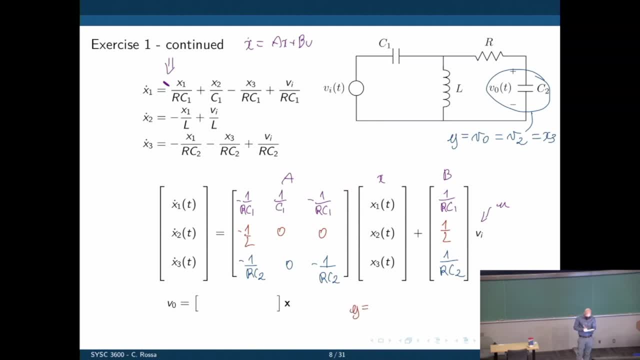 the other equation for the outputs. we want the equation to be in the form of CX plus D, U, And the equation we are trying to represent is: Y equals to X three. All right, there is no input to VI. It doesn't affect the output directly. 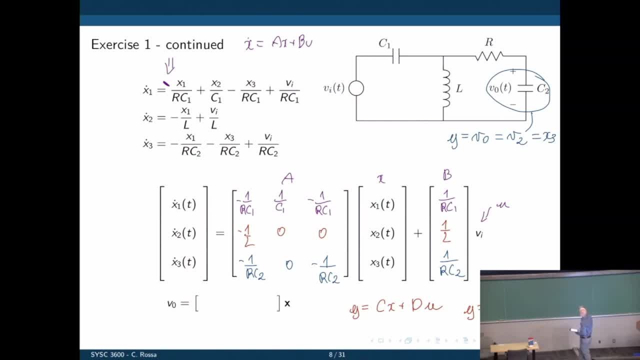 And that's pretty much it. So D is zero, D is zero. And what goes in C Here? what goes in the matrix in the vector C? What coefficients go in there? We are trying to represent this equation: Zero, zero one. 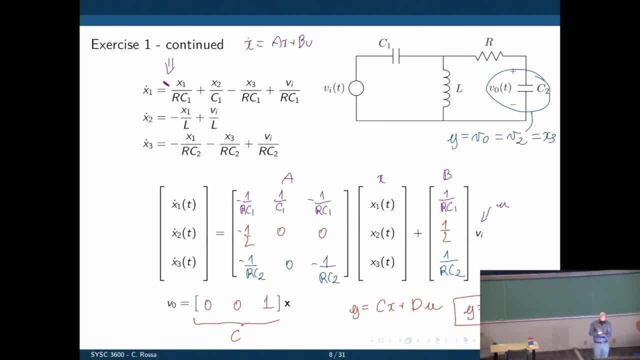 Yeah, Zero, zero, one. All right, remember that X here is X one, X two, X three. So you're going to have zero times X one plus zero times X two plus one times X three. I wish it was X three. 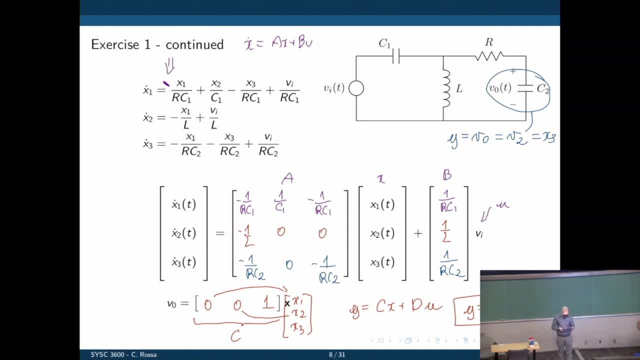 And that's our output equation. Okay, Any questions? Any questions from folks at home? You can type them or you can speak and you hear you here. No questions, all good. Now this might at first glance look a bit complicated and overwhelming. 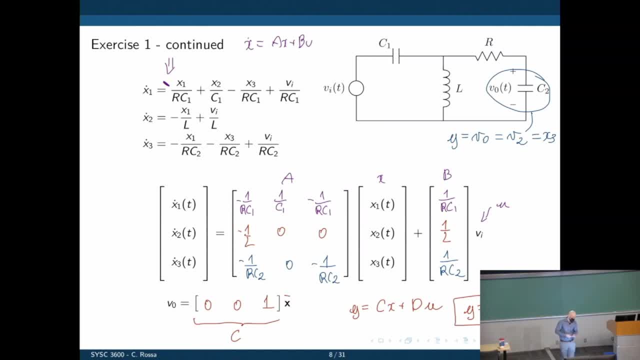 but as you do the examples, you'll see that's always the same procedure And you get an idea of how to go about finding these equations, looking for the equations. So my recommendation once again is, before we even start to writing the equations,